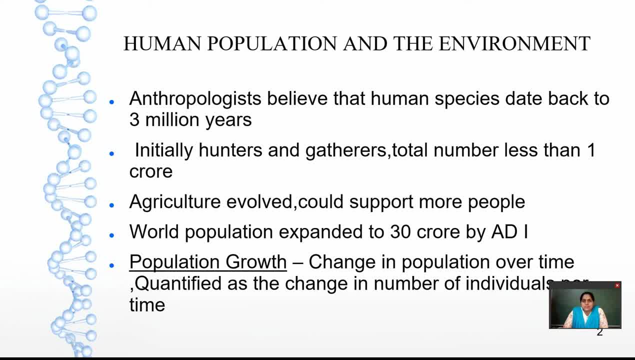 back to 3 million years, That is, you can see the human population on this earth or on the surface of the earth since 3 million years. Initially we were hunters or gatherers, That is, we used to hunt down animals or we used to- what do you say? we used to kill animals. 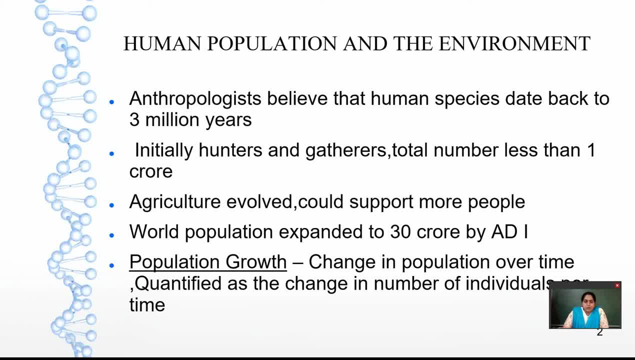 or we used to depend entirely on the forest for our livelihood. So at that age, or at that time or during that period, the total number of people or the total population of human species was less than 1 crore. because this kind of habitat or this kind of lifestyle. 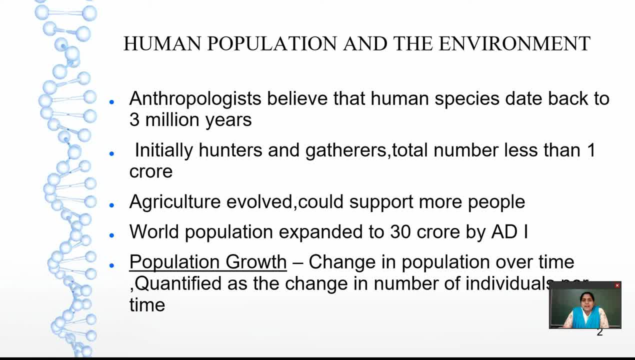 was a little difficult, because searching for food and hunting for food is a little difficult. So as a result of which, the population then was a little lesser, that is, it was around 1 crore. But later on what happened is: agricultural developed, we started developing new methods. 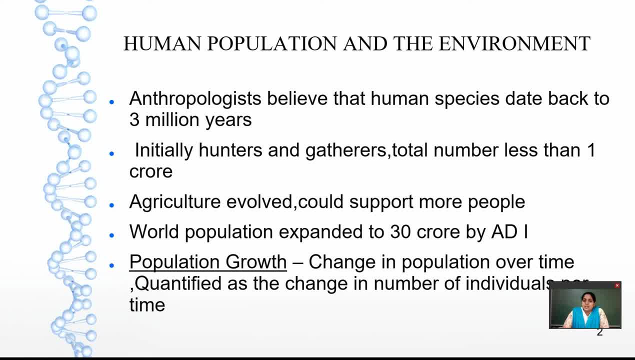 of cultivating food, So there was more food that was available. So, as a result of all these benefits that we got, the population expanded and it could support more people. So as a result of which, the population suddenly increased to about 30 crores by 81. That is. 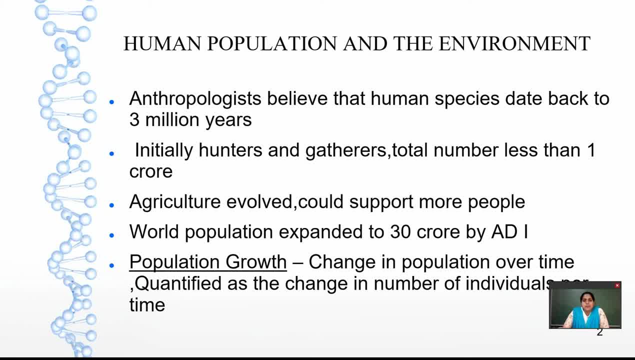 there was a sudden increase or sudden double or tripling of population. that was seen by 81.. Now coming to population growth. what do we mean by population growth? We mean by population growth: Population growth is nothing but the change in population over time. that is, how much the amount of population has changed, or what are the number of species. 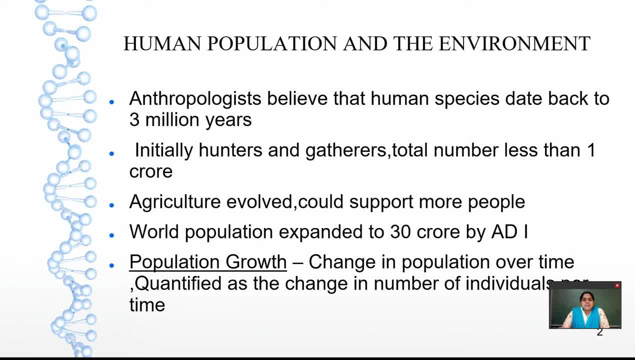 that have increased over the time And it the quantifies as a change in the number of individuals over a particular time. That is, when you are talking about population growth, you are always talking about a specific period of time. So in that period of time, what is? 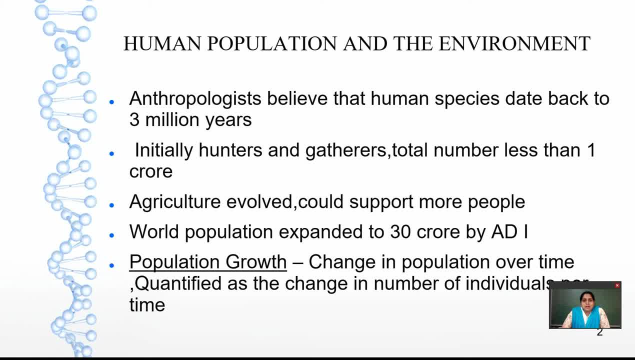 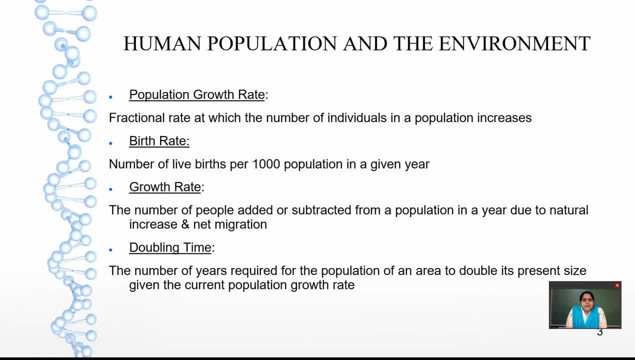 the increase in population. what is the number of population that have increased or added on to? it is what you call as the population growth. Now, coming to population growth rate, that is nothing but the rate at which the population is increasing, or it is a fractional. 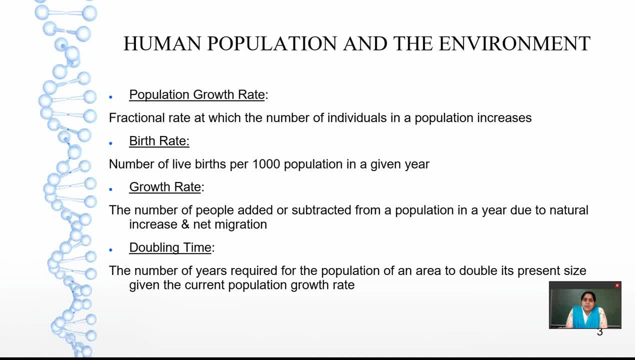 rate at which the number of individual in a population increases. So whenever you do population studies, or whenever you do studies regarding population, it is always within a specific region. That is, in that region, what is the increase in population that you see? So 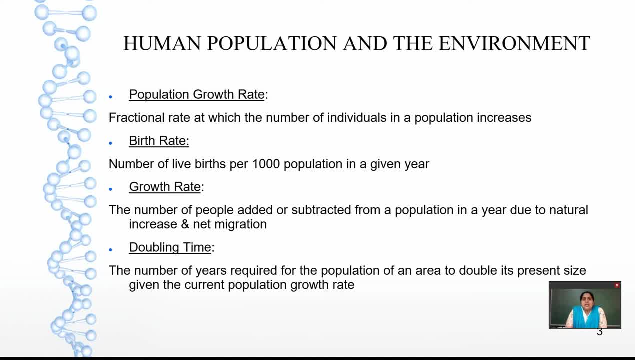 population growth rate is nothing but the rate at which, or the fractional rate at which, the number of individuals in a particular area or region are increasing. Now coming to birth rate. birth rate is nothing but the number of live births per 1000 population in a given year, That is. it is the. 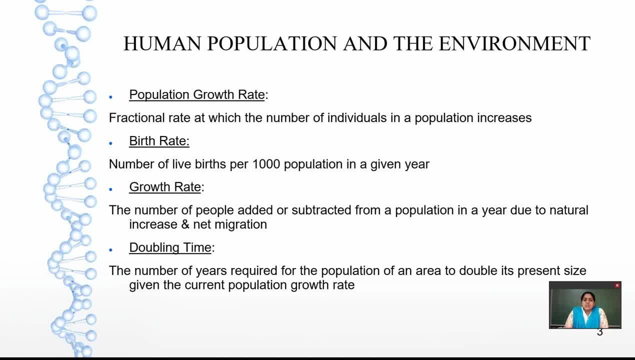 percentage, calculated considering 1000 individuals. So what are the number of births which are happening per 1000 individuals in a given year is nothing but the birth rate of that particular region or that particular nation. Now coming to growth rate. what is growth rate? Growth rate is? 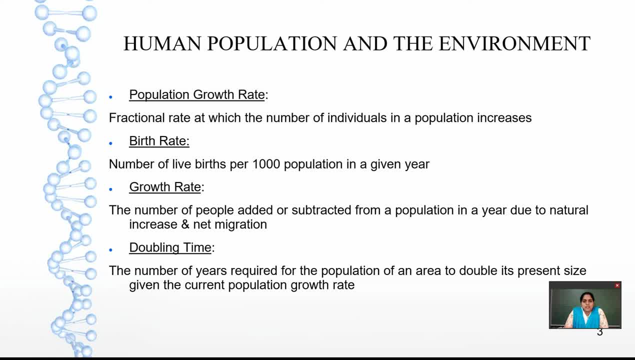 the number of people that have been hydrated or subtracted from a population in a year due to natural increase or net migration. Now, birth rate is basically the number of births which have happened in a year. Now, birth rate is basically the number of births which have happened in a 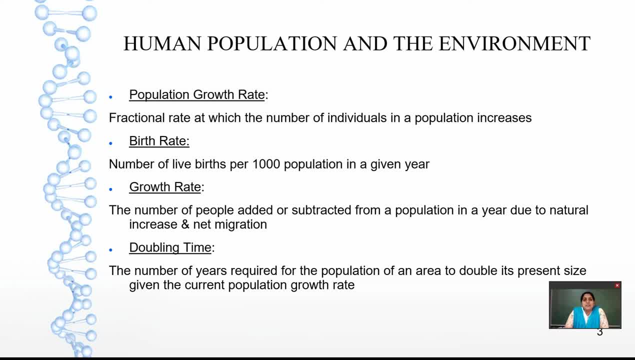 year. But growth rate basically increases, basically measures whether the population has grown or it has been decreased. That is, it can be either ways. It can be a growth in the population or growth in the number of individuals, or it can be a deletion or subtraction in the number of. 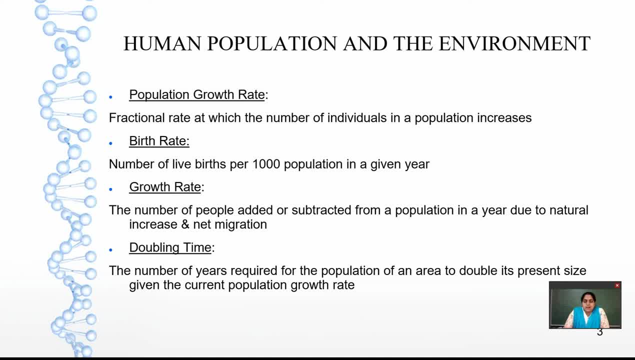 individuals Again, since, like I said, it is an area wise mapping. So, as a result of which, when you consider the growth rate of a particular area, it would have increased due to births, or it can, or due to migration, or it could have also decreased due to birth or migration, So it is to a particular. 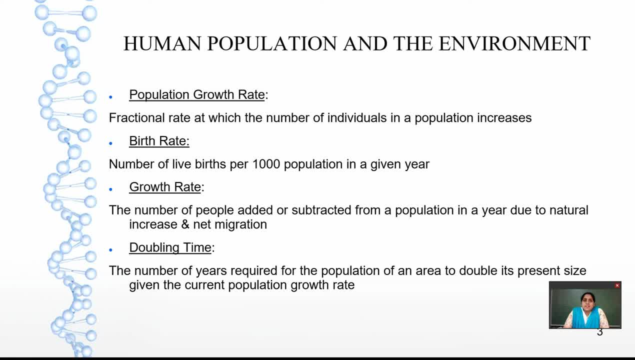 area. Now, what is doubling time? Doubling time is nothing but the number of years which are required for the population of a particular area to double its present size. That is, you are calculating the population of a particular area at one particular time. Now what will be its doubling rate? That is? 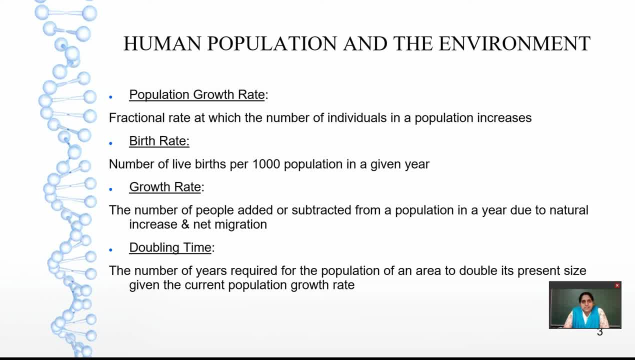 you would say what is the time taken for that particular population to double in its size or to double in its quantity for a given, in a given period of time is nothing but the doubling time, That is, how much time that particular area or that particular population takes to double its. 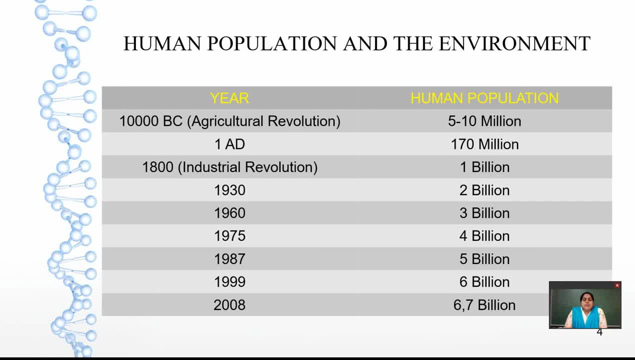 current size. Now, when you study about human population and the environment, you would see what is the growth rate or what is the increase in population that you have seen over the years. That is, in 10,000 BC, when the agricultural revolution happened, there were around 5 to 10. 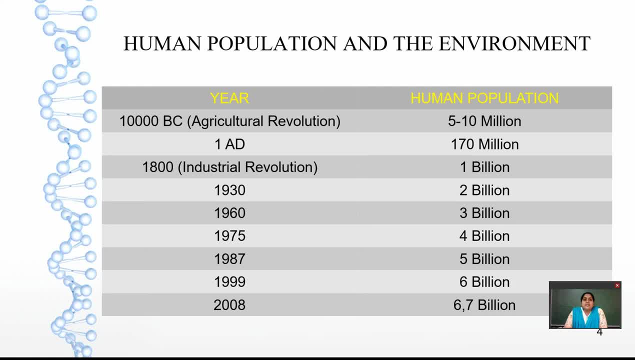 million people living on this planet, whereas in the first AD it increased to around 170 million people. Then came the industrial revolution. That is when, with the industrial revolution, there came more opportunities for jobs, better life, better livelihoods, better standards of living, So as a result of which it suddenly increased to. 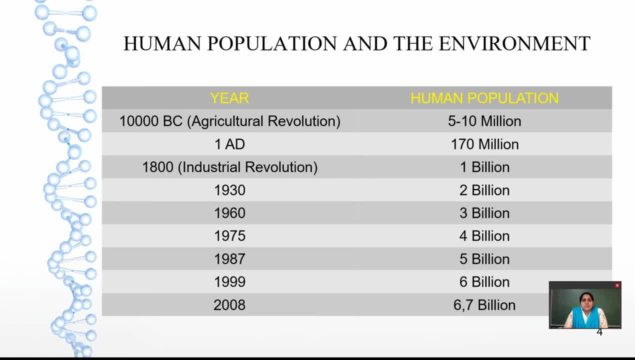 1 billion and so on. it moved on to 6 to 7 billions in 2008.. So you can see there is an exponential growth in population. that is seen with the limited resources that have. limited resources have always been limited. It is only the facilities or the benefits that we are getting in. 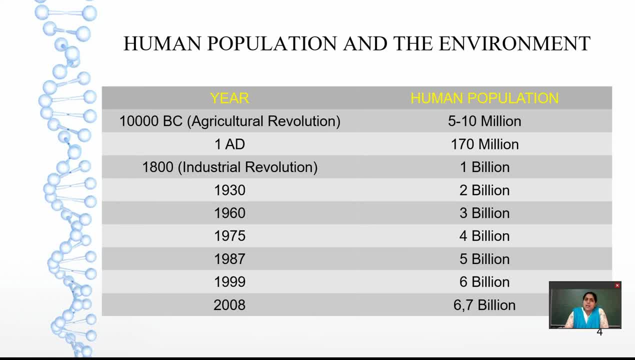 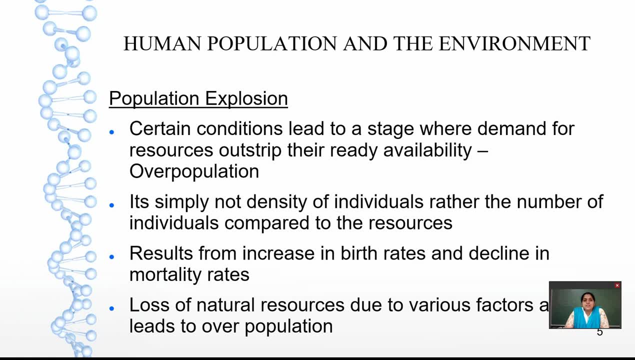 other forms, whether it is from the industries or from the agriculture, that has increased. So, as a result of it, the population also seems to increase. Now coming to population explosion. what do you mean by population explosion or overpopulation? Now, certain conditions lead. 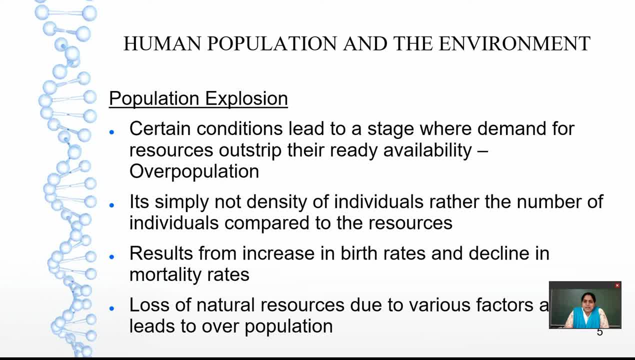 to a stage where the demand for resources outstrip their ready availability. Now, when you are talking about population explosion, you should not only talk about not only the number of people who have increased or number of species that has increased. you should also talk. 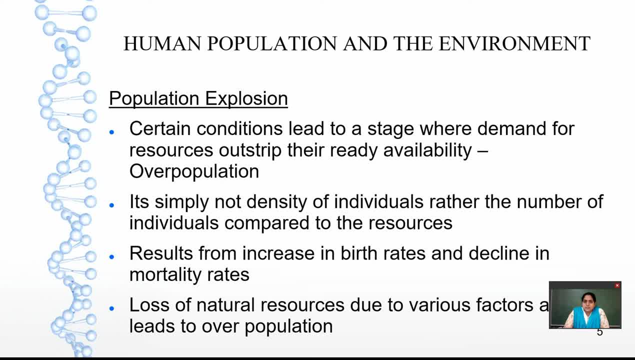 in terms of proportion, That is, to the number of available species which have increased. what is the amount of available resources? That is, it is always an interconnected factor. That is when you are talking about population explosion. what do you mean by population? 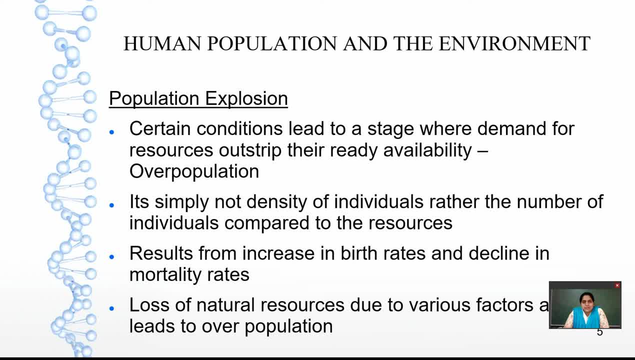 explosion. You should not only talk about the number of species that have increased. you should talk about whether the resources are available for those particular species. If the resources is less, that means the population is more. If the resources are equal or enough for the entire. 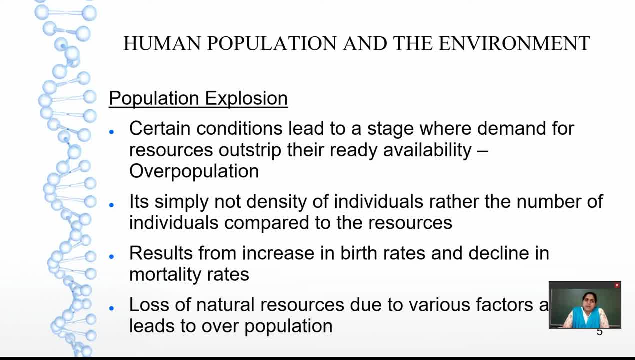 population. that means the population is stable or it is under control. So overpopulation is nothing but where the demand for resources outstrip their availability. That is, where the demand is more but the availability is less. Such a condition is called as overpopulation or population explosion. 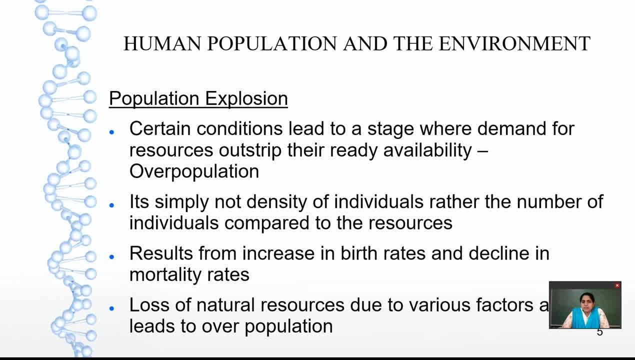 Now it is simple: not the density of individuals, rather than the number of individuals which are compared to the resources. Again, it is not the entire density of the population which is taken into consideration here, but whether the resources are available for the individuals. is what we are. 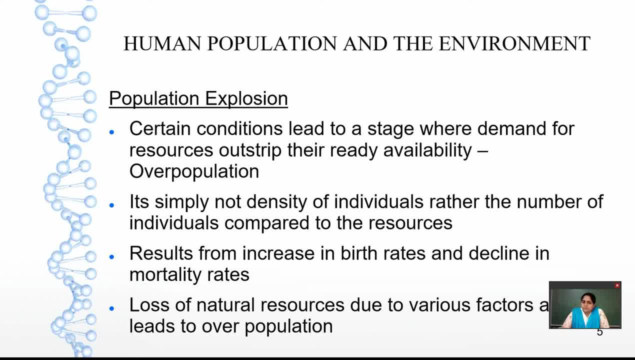 taking into account here Now the results from increase in birth rates and decline in mortality rate. So how does population explosion occur or how is there? overpopulation is nothing, but it is due to increase in the number of births. So it is not the number of births, it is the number of. 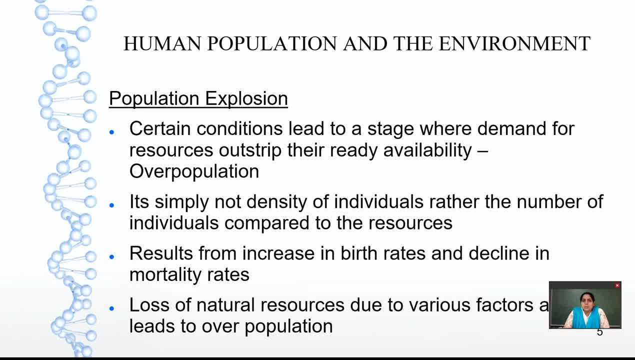 birth rates and decline in the death rates. So this is a simple logic that you can apply. how is the population increasing? because the number of people who are being born are more, there is a number of people who are dying or the mortality rates are lesser comparatively. 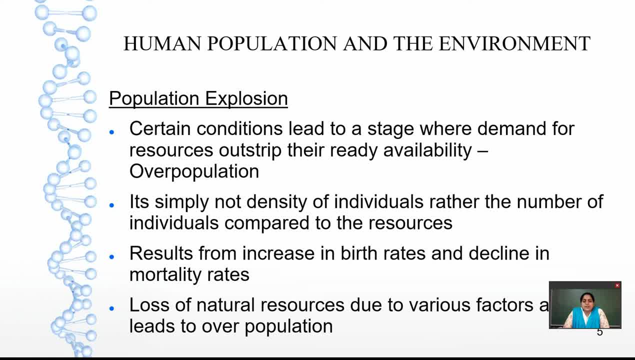 Now, loss of natural resources due to various factors also leads to overpopulation. So overpopulation cannot only be due to the increase in birth rates, but it can also be due to the declination or degradation of the natural resources, which can be brought about by 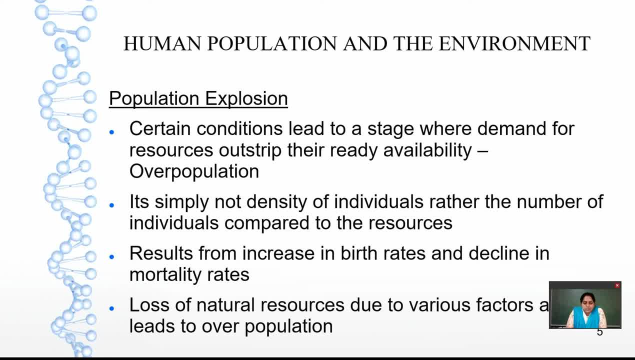 various factors, like we have discussed in the previous chapters. It can be due to natural factors, it can be due to manmade factors and all that. So depletion of natural resources also. what is happening is, since the natural resources are depleting the amount that is available for. 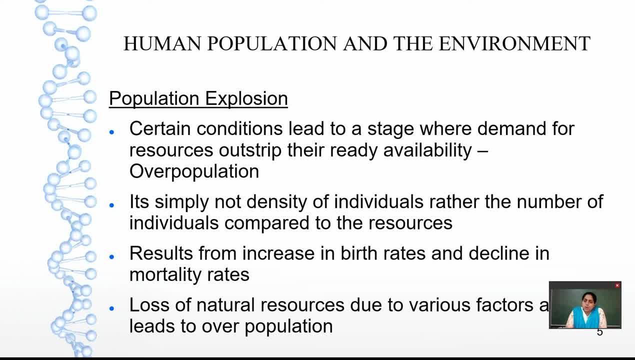 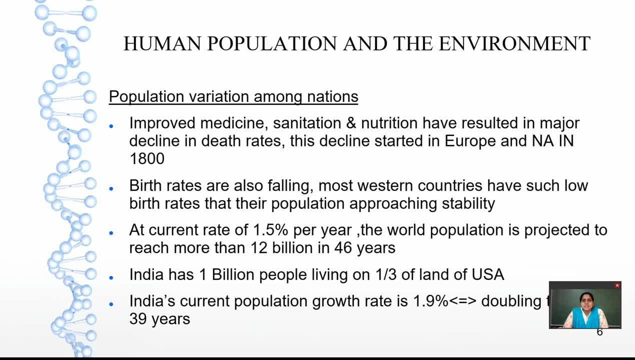 the population is also lesser So, as a result of it, you can consider it as overpopulation or population explosion. Now coming to population variation among the various nations, that is, what are the, what is the population rate or what is the growth rate in the various nations? 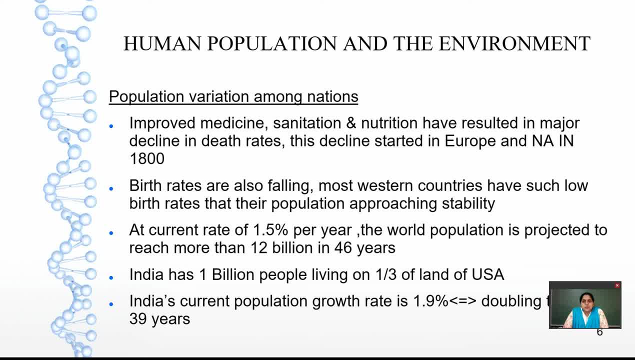 You see that improved medicine, sanitation and nutrition have resulted in major decline in death rates. This decline started in the Europe and North America Now earlier. what used to happen is people used to die a natural death. That is because of the various diseases that they 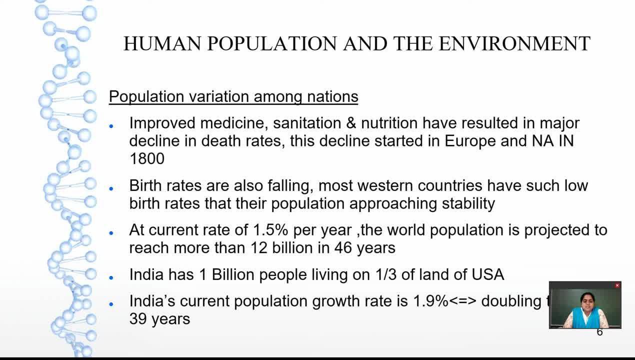 had, or due to aging or whatever it is. they used to have a natural death. So as a result of it, there was a balance between the number of people who were born and the number of people who died. But in recent years we have come up with newer medicines- anti-aging medicines, or it can be. 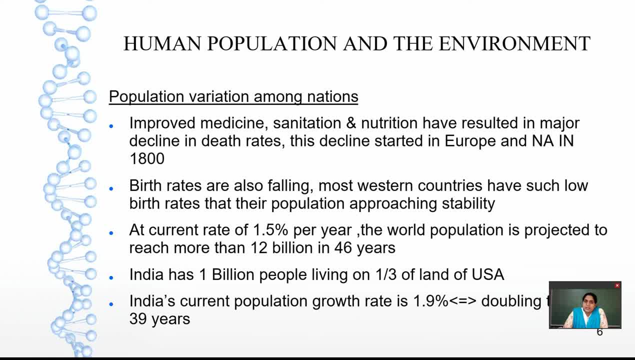 medicines which can cure deadly diseases, which were not there initially. So as a result of which the mortality rate has decreased, That is, the people who number of people who are dying, who die, have decreased. So as a result of which, in the developed countries like Europe and North, 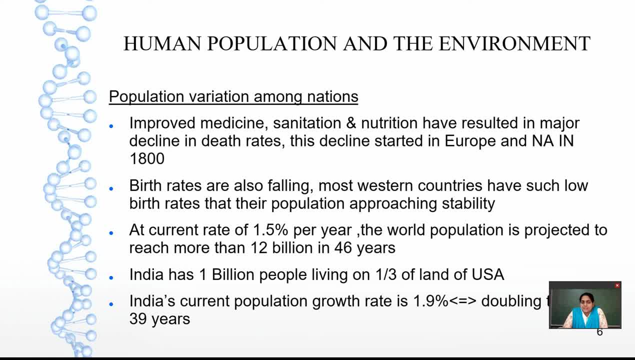 America, etc. their population explosion is seen to a certain extent. Birth rates are also falling. Most western countries have such low birth rates that their population are approaching stability. Now there is another phase to this. also There is there is population explosion on one side. 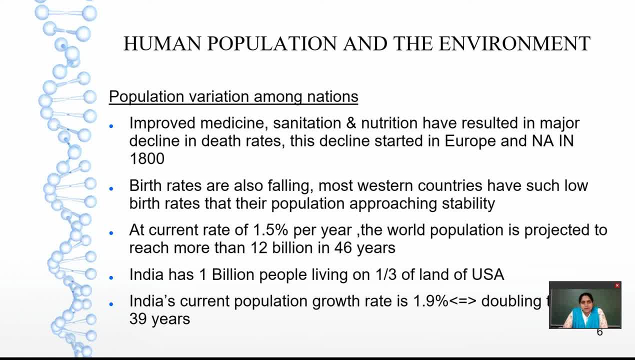 but there is also a decrease in the number of birth rates, also in some countries. So, as a result of which, what is happening is newer generations are not getting added on, It is only the older generations which are passing on, So, as a result of which, the population of that 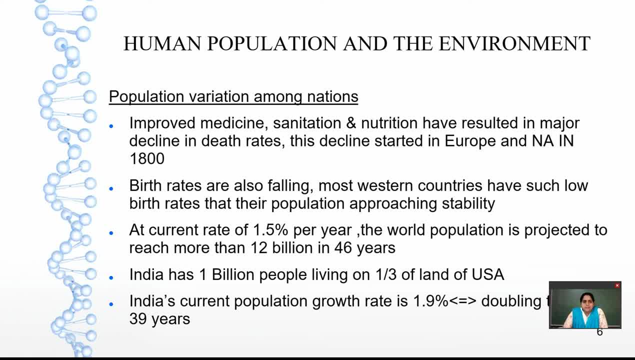 particular nation, where the birth rates are low, is stable Now, in the current rate of 1.5 percent per year. the world population is projected to reach more than 12 billion in 46 years. That is given the data that that human growth rate, or the growth rate of humans, is around 1.5 percent. 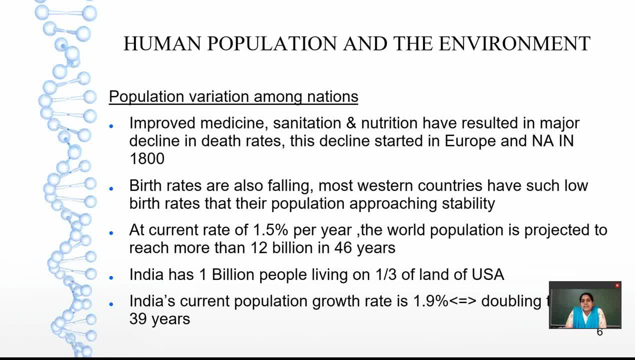 per year. it is estimated that we can. we will be reaching the total population of 12 billion in 46 years. Now India has 1 billion people living on one-third of the land of USA. Now India is called as overpopulated, again because the resources which are available in India are 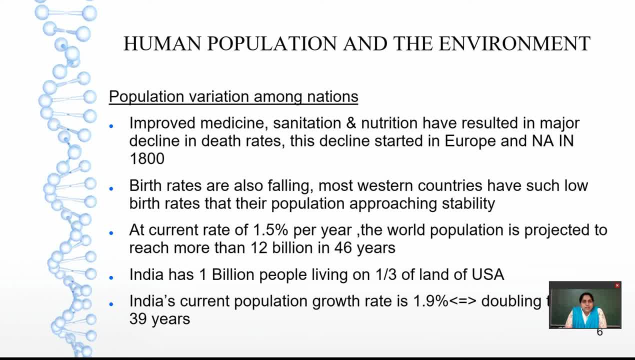 not enough, are not sufficient to fulfill the needs of the population. Now there are around 1 billion people in India, and all of them are living in a area which is one-third of USA. That is, the total area of USA is much, much larger than that of India, but the population 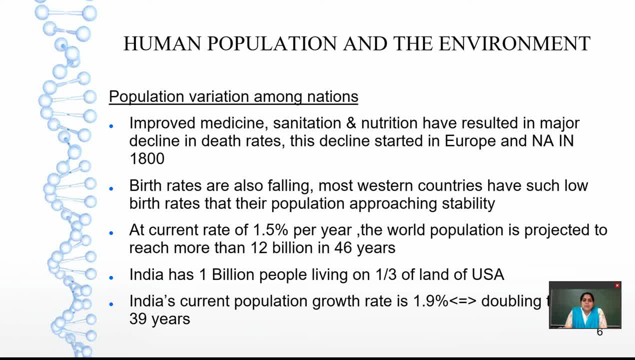 of India again is larger than that of USA. India's current population growth rate is around 1.9, see, when you talk about the growth rate of Indian population, it is around 1.9 percent per year. that is, growth rate is increasing by 1.9 percent per year, which is equivalent to a doubling year. 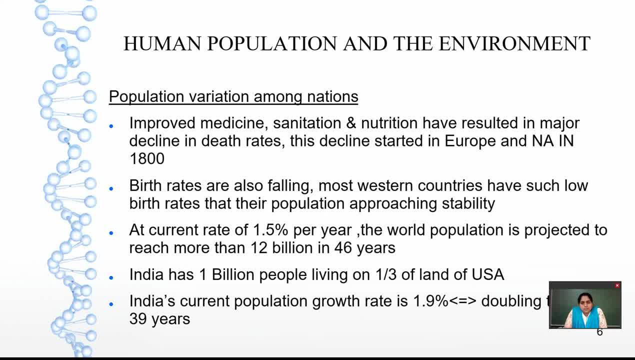 of 39 years. That is when you talk about, you know, doubling rate. that is, you would say the population would double in another 40 years or 50 years, or whatever it is. When you are considering India's current population, you see that the growth rate is around 1.9 percent. So, as a result of which, 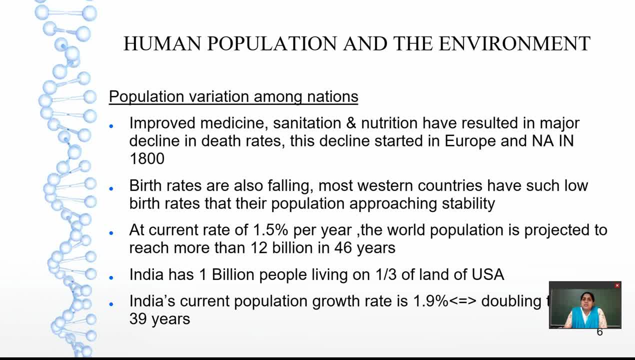 since it is increasing exponentially in 1.9 percent per year, so, as a result of which the doubling time or the doubling rate has decreased, and then the population will be doubled within a mere 39 years. itself okay, The population will be doubled, the size that it is now within. 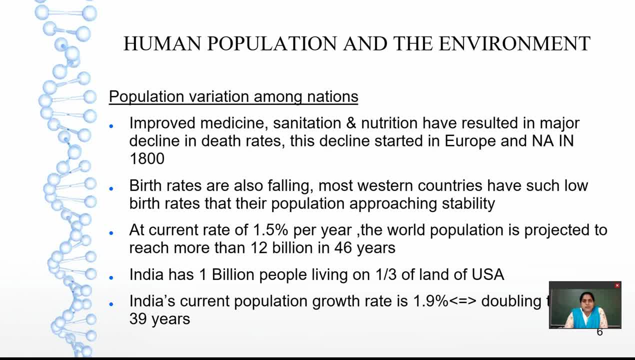 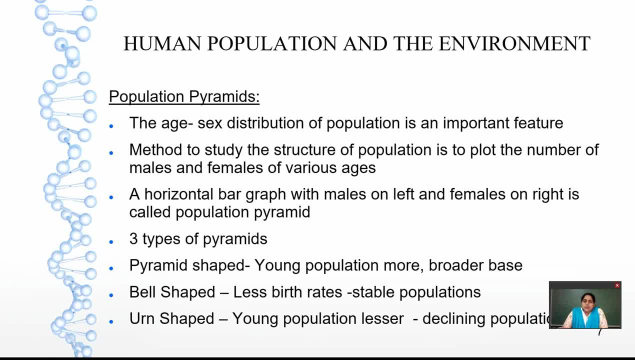 39 years itself, which is a very, very small period, or very, very small doubling rate. Now, based on the data that is provided, or based on the data by the researchers, you can construct something called as a population pyramids, The population pyramid basically. 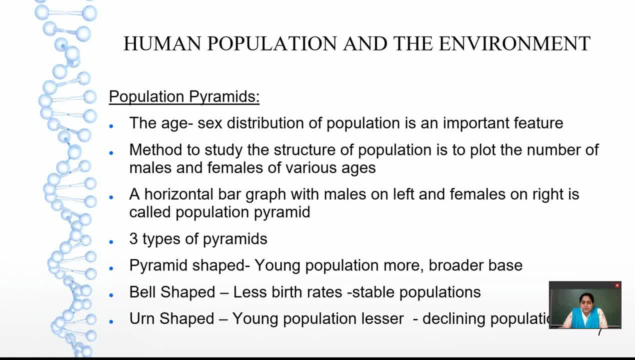 is nothing but the age. sex distribution of population in in any is an important feature of these population pyramids. that is based on males and females, and what are the ages of the males and females which are present in that particular population? will give you the population pyramid. Now, the methods to study the structure of population is to plot the number of males and 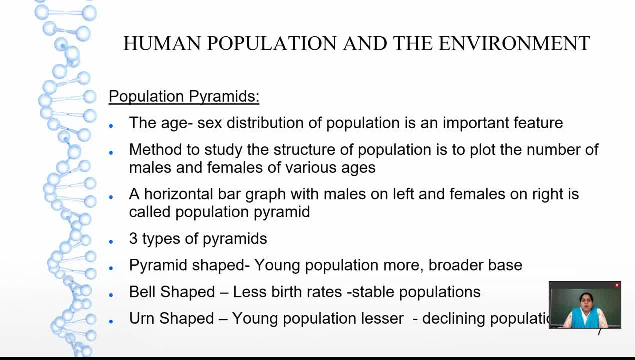 females of various ages. So how does this population of pyramid built up, or how is a population pyramid form? It is nothing, but you are plotting the ages of males and females in that particular population and thereby building the population pyramid. So this is a very, very 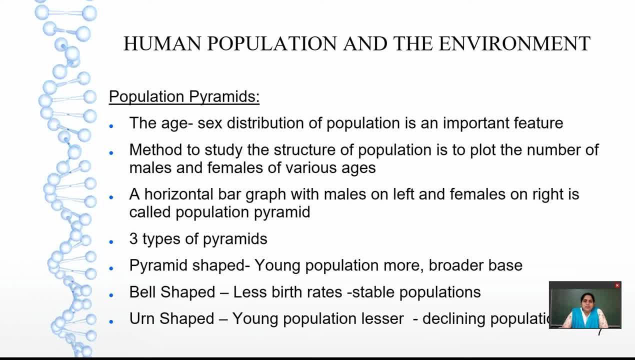 within the pyramid, A horizontal bar graph with males on the left and females on the right is called as a population pyramid. So in the population pyramid you have the males on the left with their ages and you have the females on the right with their ages. 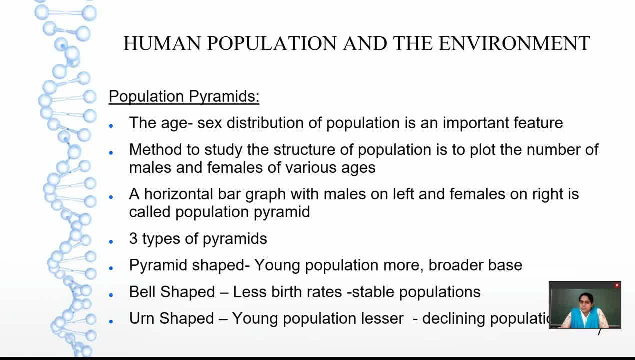 Now, depending on the population, there are three types of pyramids which can be formed. You have the pyramid-shaped population pyramid, wherein the younger population is more so, as a result of which, since you are plotting it against the age of human beings, so the 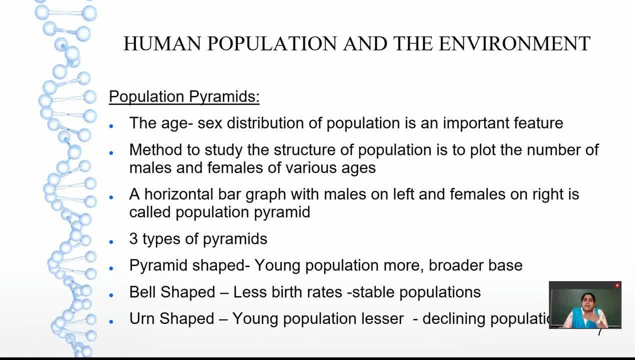 base will be broader, whereas the top will be lesser, because here the younger population is more, So that will form a pyramid-shaped population pyramid, Coming to bell-shaped population pyramid. what is happening here is the birth rates are lesser in such countries- See young population- where the young population is more, forming a pyramid-shaped population. 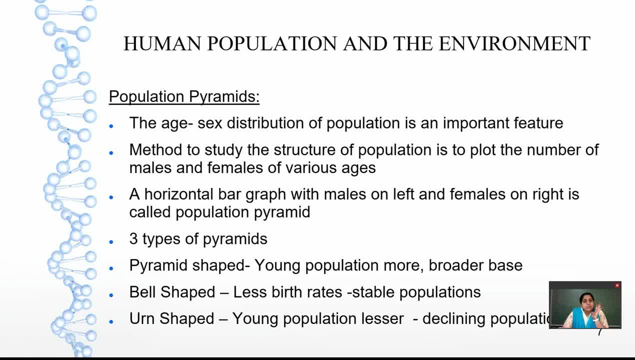 pyramid. Example is India, Bangladesh, all these regions where the birth rates are higher, So as a result of which younger generation or the number of younger generation is higher, Whereas in bell-shaped population pyramids what is happening is there are lesser birth. 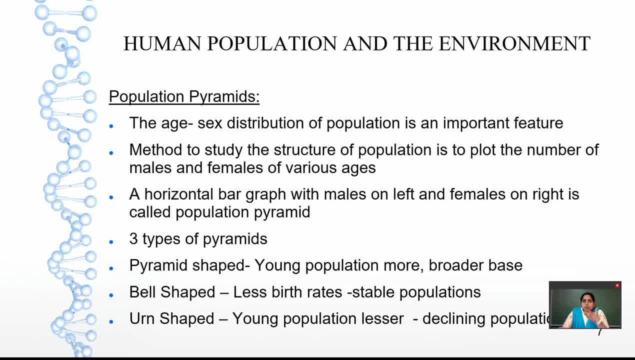 rates, That is, there are lesser- what do you say? number of people who are being born. So, as a result of which, the older population, as they pass on, like we told previously, form a stable population, Coming to urn-shaped population pyramids, and so, in urn-shaped popular pyramids, the younger 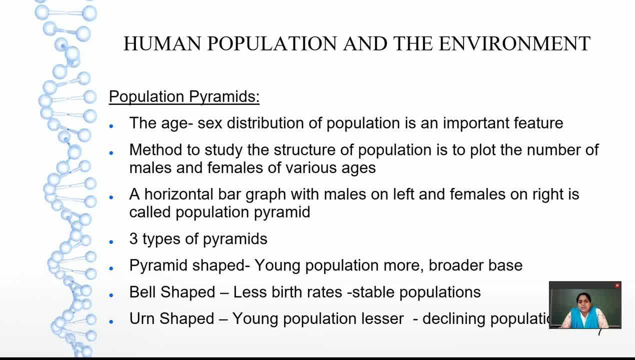 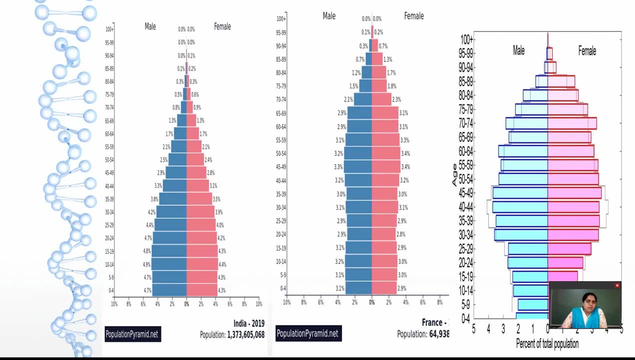 population again here is lesser and there is a declining population, That is, the number of people who have reached the mortality age, or the age of where they're about to die. So, as a result of which it forms an urn-shaped pyramid. Now, these are the graphical representations of pyramid-shaped and bell-shaped as well. 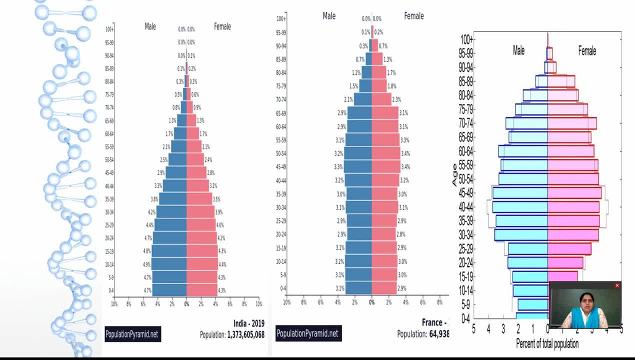 as an urn-shaped population pyramid. Example for bell-shaped population pyramid is nothing but France, where the older or the people who are in the middle age are higher, Whereas the example for an urn-shaped pyramid is Germany, etc. where you can see the people who are who have crossed the reproductive age are much, much higher, or the number of 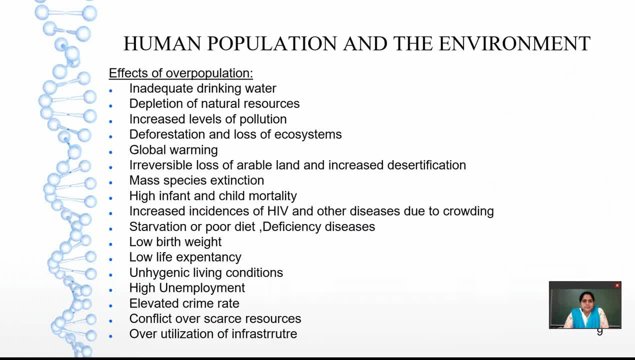 people who are in the, who have crossed the reproductive age, is higher. Now coming to what are the effects, or negative effects rather, of overpopulation? That is, what are the? what is, how is overpopulation affecting us? why are we today studying overpopulation? all this, if we are going to study now. 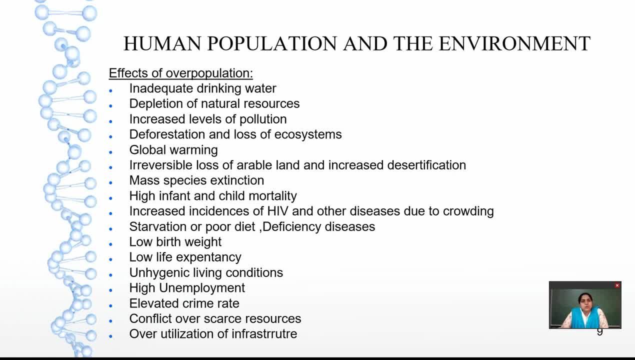 That is because of overpopulation, there will be inadequate drinking water. So, as we told, resources, but one of the most important resource, or the main resources that are required for the survival of human life, The survival of human beings, is nothing but drinking water. Now, there will be inadequate drinking water if there is overpopulation, that is, it will. 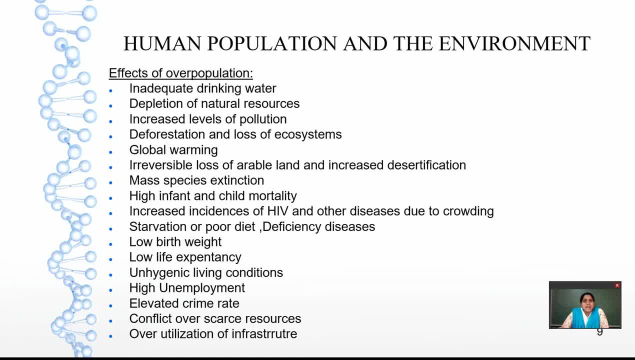 not be enough to feed everybody As of it. as of now, only, we are paying for water. okay, water, which used to be free in our younger days, rather, is something that we are paying for now, So, as a result of which, it is indicating that we are already on shortage of water. 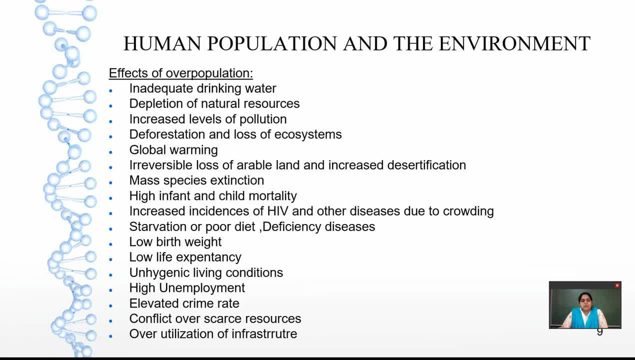 So overpopulation will only lead to more inadequacy of drinking water. Depletion of natural resources, of course, because we are using more and more resources. as the population is increasing, we are already using a greater number of resources. as a result of it, there will be a depletion in the natural resources. 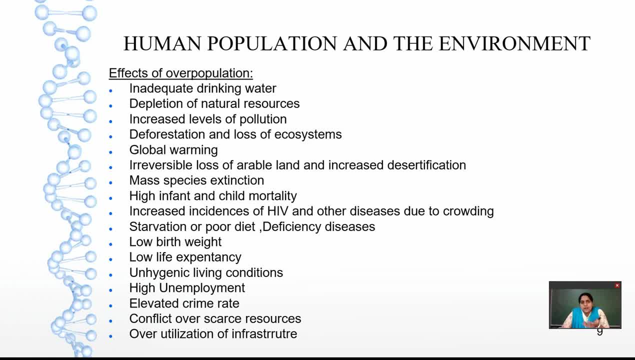 Increased levels of pollution. that is because we are- see, all of us today, we are all very lazy to walk or to go by bus, or to go by a or to go on by any kind of communal transportation. We go, we go in for individual vehicles, whether it is two wheelers or four wheelers. 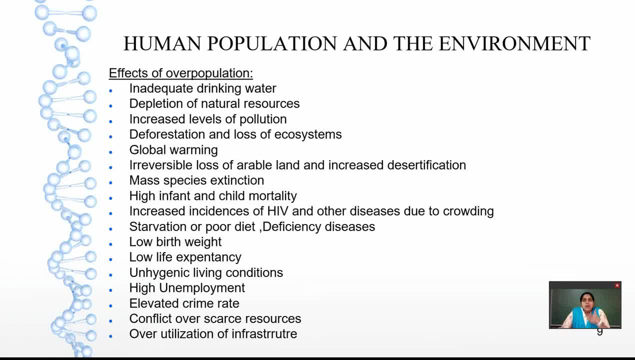 So what we are doing, we are only adding to the pollution in the environment. So more people, that means more pollution is added into the environment. So what we are doing, we are only adding to the pollution in the environment. So more people, that means more pollution is added into the environment. 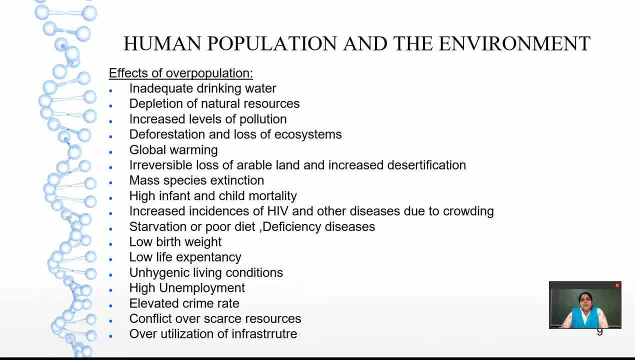 Okay, Deforestation and loss of ecosystems. Deforestation and loss of ecosystems Again, where will you accumulate all these people? everybody needs a new home, everybody needs a new villa. So, as a result of it, what you are doing is you are clearing up the forest. you are clearing 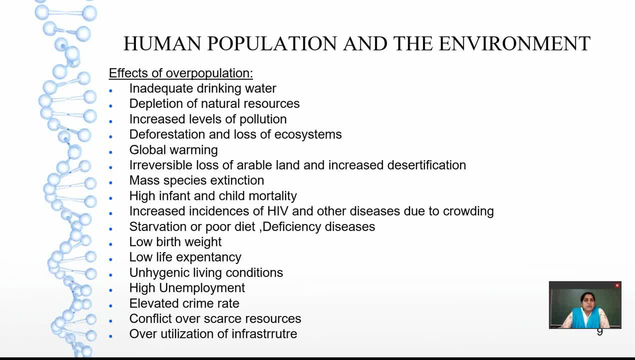 up the other kinds of ecosystems in order to create spaces or in order to build apartments. In Bangalore, what is happening? they have closed the rivers or the lakes and they have built apartments on these lakes. So you are closing down or you are losing those ecosystems. 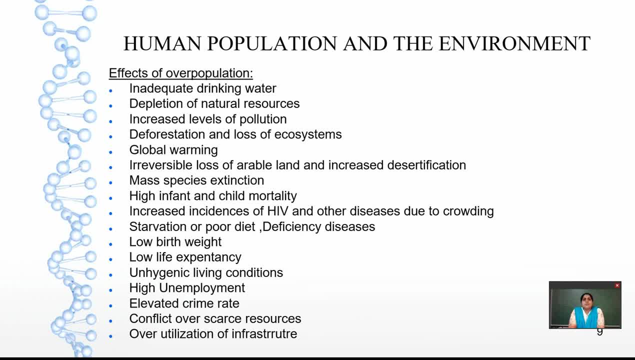 Of course global warming because we are emitting the greenhouse gases. Of course global warming because we are emitting the greenhouse gases And thereby bringing about global warming. it is again us humans, again. the reason for this is very much overpopulation, Irreversible loss of arable land and increased desertification. 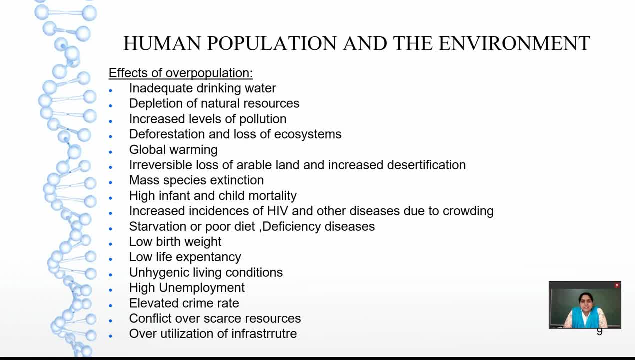 Irreversible loss of arable land and increased desertification. That is what is happening because, in order to clear up, we are not giving importance to agriculture anymore, Even though it is one of the main reasons that we are surviving today. it is one of 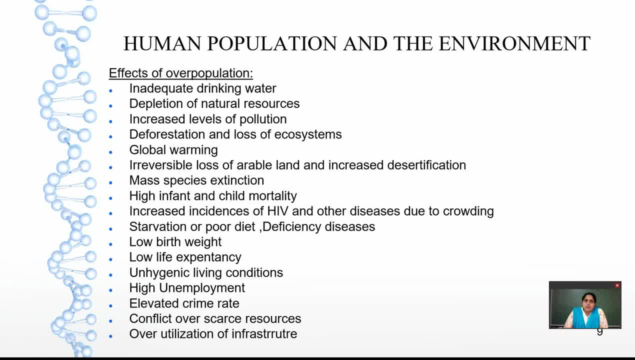 the sources of staple food, but still we are not giving importance to agriculture. We are clearing off the agricultural lands and going in for monocultural plantations in villages, or we are going for commercial complexes in villages, Okay, Okay, the urban areas: Mass species extinction again. when there is a loss of habitat, when the loss of 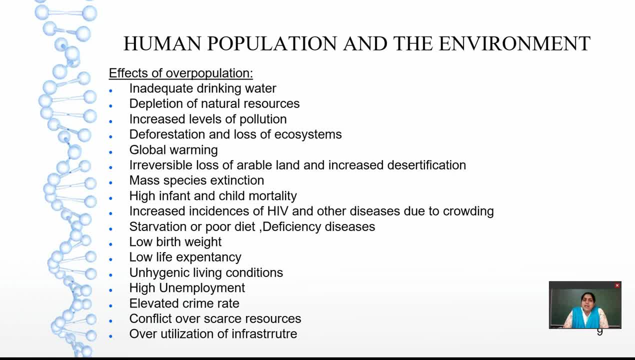 the, when the habitat of that particular area is lost, what is going to happen? There is going to be a species extinction. that is, species which could be seen earlier, were not, will not be able to see in the future High infant and child mortality. that is again because of overpopulation. 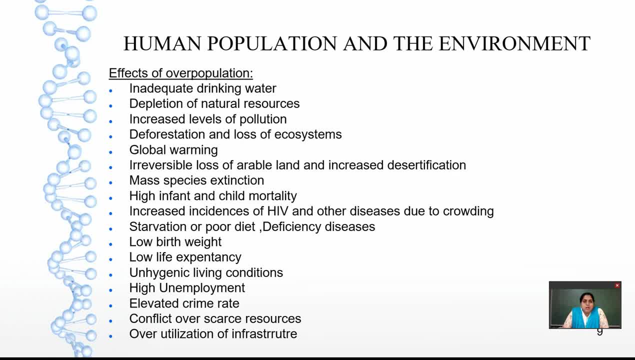 you are without thinking. you are giving birth to new individuals again. there will be a lot of problems in them, lot of diseases may be seen so, as a result of which there will be high infant and child mortality because you are bringing them into such polluted environments. then the infant- 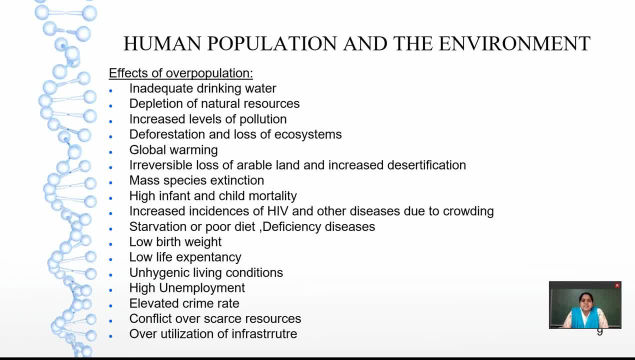 mortality has increased in the recent years, Increased incidence of HIV and other diseases due to crowding again, HIV or any such endemic diseases- sorry, epidemic diseases are the ones which can be transferred from people to people, so as a result of which, as the population increases, 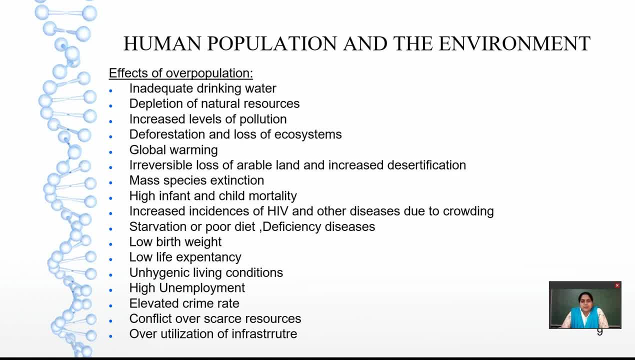 there is a chance that such epidemic diseases also are transferred to a huge number of people: Starvation or poor diet deficiency diseases, of course, when there is, when the natural resources are depleting, the food sources are also depleting, so as a result of which, less